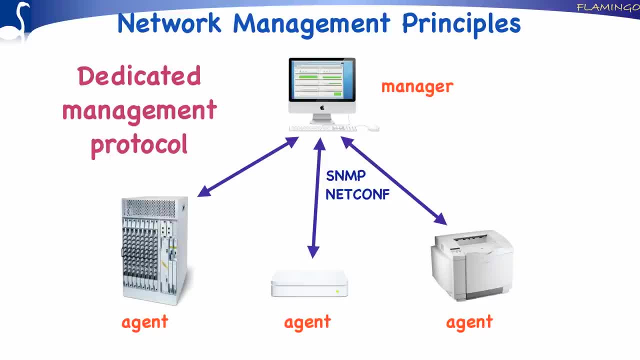 At the same time that SNMP was being developed, the International Standardization Organization worked on defining CMIP, the Common Management Information Protocol. This protocol has, amongst others, been used for managing mobile telecommunication networks. Yet another approach is WEBM- Web-based Enterprise Management. 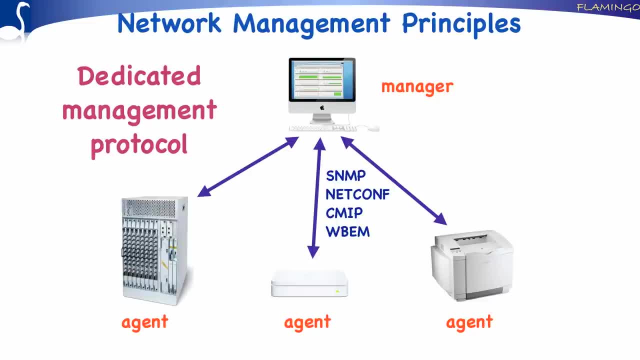 WEBM is developed by the DMTF, the Distributed Management Task Force, and supported by various operating systems. A special kind of management protocol is Syslog, which allows the agents to signal certain events to the manager. Syslog has been implemented within UNIX systems since the 1980s. 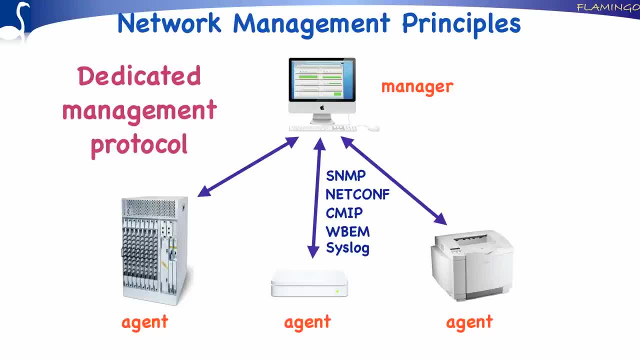 and is nowadays standardized by the IETF as well. One of the tasks that managers perform is to monitor specific management data, such as the number of packets dropped on a specific interface. To retrieve such management data from the managed device, the manager uses a GET REQUEST- PDU. 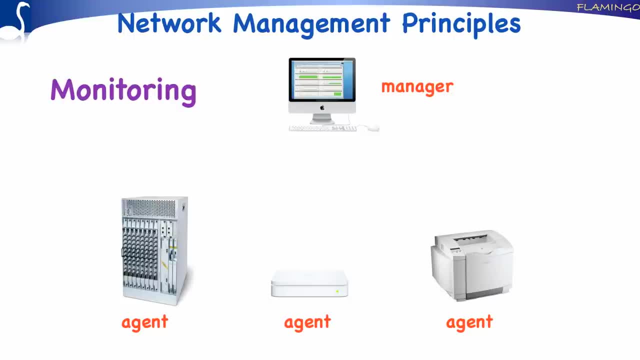 After reception of the GET request, the agent retrieves the requested information from within its device and sends this information back to the manager via the GET RESPONSE PDU. Another task that managers can do is to configure a device by setting certain management variables, such as an entry in the forwarding table. 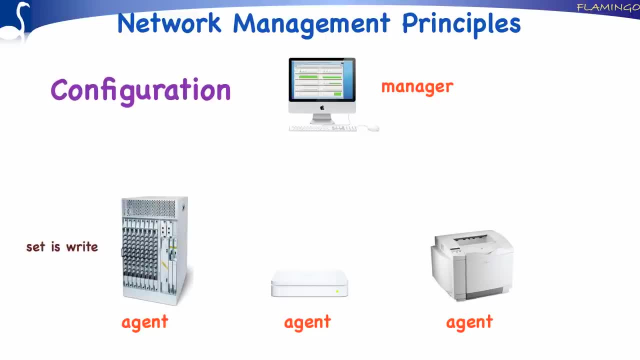 For that purpose, the manager sends a so-called SET PDU to the agent. Finally, agents may be able to autonomously signal certain events to the manager, for example in case an interface went down or the device has been reset In the first version of SNMP. 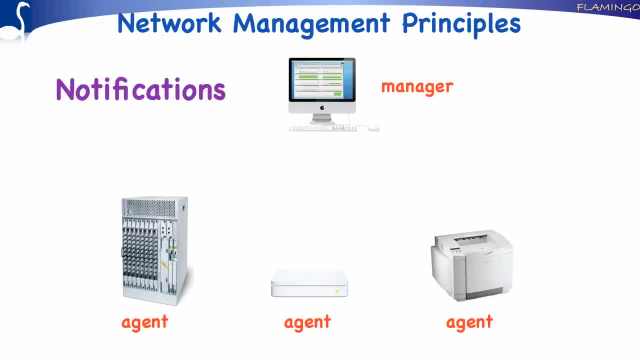 agents could signal only a limited number of events to the manager using the TRAP PDU. In later versions of SNMP, the capabilities for agents to notify all kinds of events have been extended. For that purpose, a new PDU was introduced, the INFORM PDU. 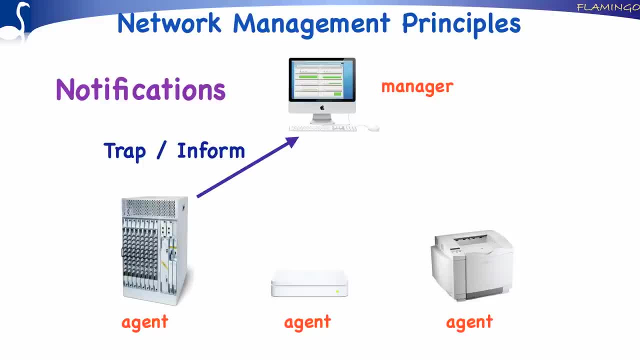 which is acknowledged by the manager. so the agent knows the manager is aware of the event. Let's now focus on SNMP, which is the most important management protocol for the Internet. An important goal during the early development of SNMP was to keep the implementation of agents as simple as possible. 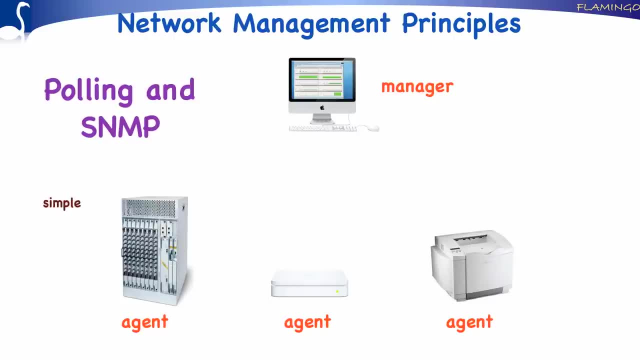 Agent functionality therefore remained limited and, as we have just seen, agents had only minor capabilities to monitor their own behavior and notify the manager in case of problems. As a consequence, the manager had to continuously poll the agents to learn their status using GET, REQUEST PDUs. 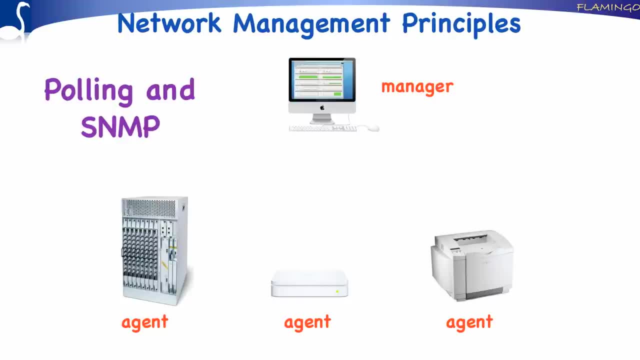 It is interesting to compare this philosophy to keep agents as simple as possible to the philosophy behind CMIB. In the case of CMIB, agents should be quite powerful and able to autonomously inform the manager in case of problems, As opposed to SNMP. 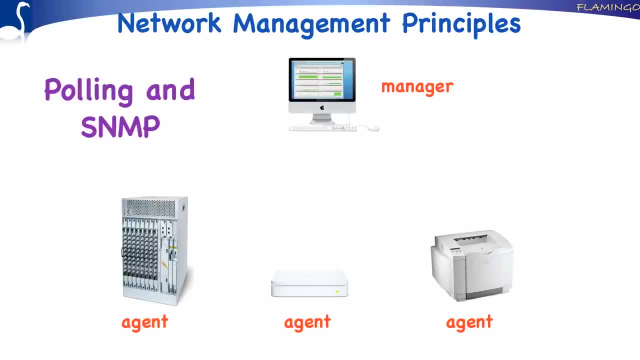 the implementation of CMIB managers should therefore be relatively straightforward, As discussed before. after reception of the GET PDU, the agent retrieves the requested information and sends this information via the GET RESPONSE PDU back to the manager In case polling is performed sequentially. 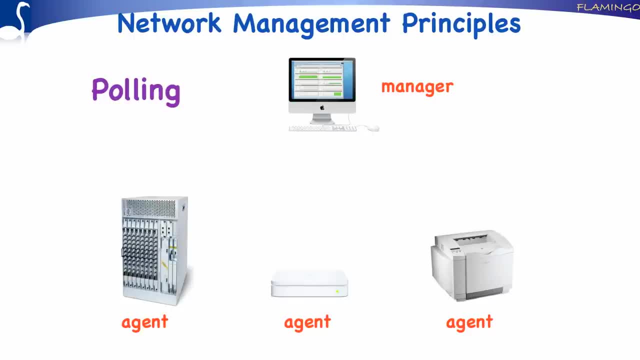 the manager will now poll the second agent And also this agent reacts by sending a GET RESPONSE PDU. Depending on the amount of information being requested, it generally takes in the wrong order. For instance, the manager may have to take an order of milliseconds. 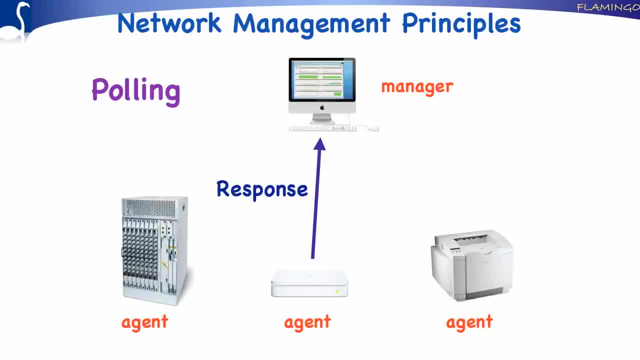 to retrieve that information from within the managed system and send the response: PDU. There are agents, however, that have rather poor agent implementations and need hundreds of milliseconds or even seconds before being able to send the response. In our example, the manager now polls the third agent. 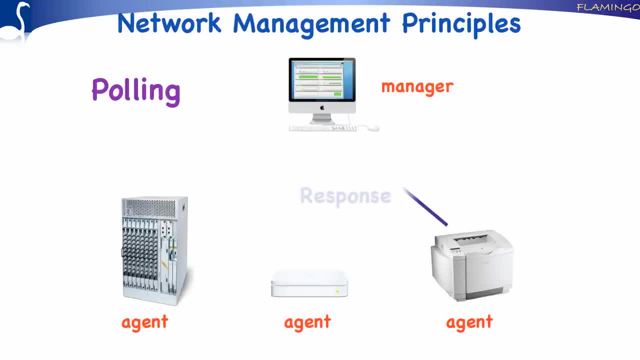 But in case of larger networks the manager may have to poll thousands of agents. Since polling may take quite some time, the span of control for a single manager will be limited. In addition, the manager will have to handle a lot of management traffic. 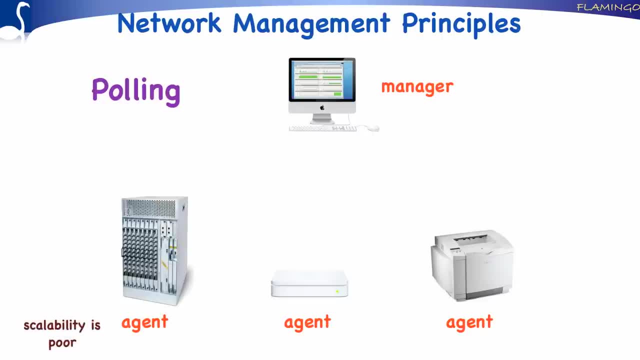 Scalability is therefore poor and if thousands of devices need to be polled, the tasks of the manager should rather be distributed over several managers. To distribute the management functionality of the original manager, a hierarchy of managers can be created In such hierarchies. 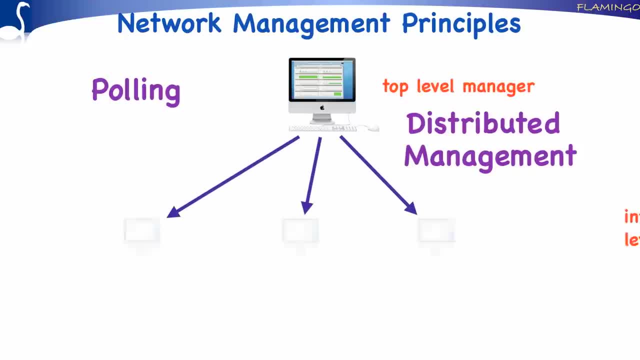 the top-level manager interacts with the intermediate or mid-level managers which, in turn, poll the various agents. Intermediate-level managers may be tailored to the polling of one specific type of agent, such as all routers, or generic for all kinds of agents Within the IETF. 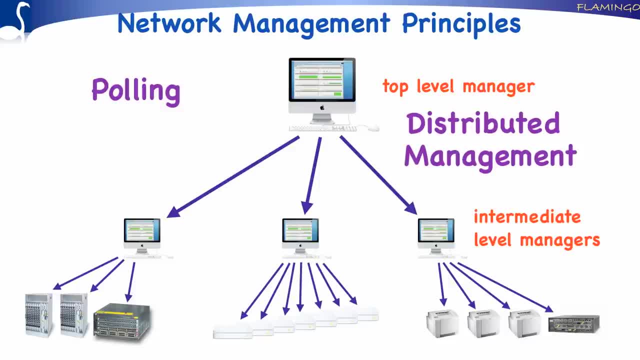 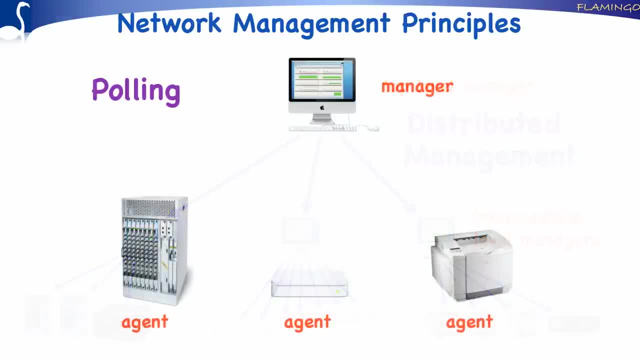 the protocols and information for such management hierarchies have been defined by the distributed management – this man – working group. Instead of sequentially polling all agents, the manager can of course also poll all agents in parallel. Care should be taken, however, to not generate too much management traffic. 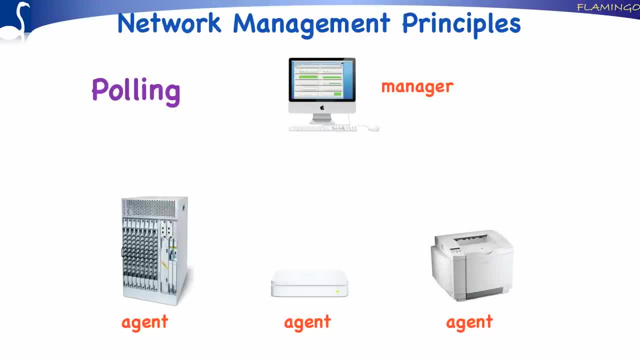 at the same time, And, of course, we have to poll all agents again after a certain period, which is often a five-minute interval. Polling goes on 24 hours a day and will therefore be responsible for the major share of all management traffic. 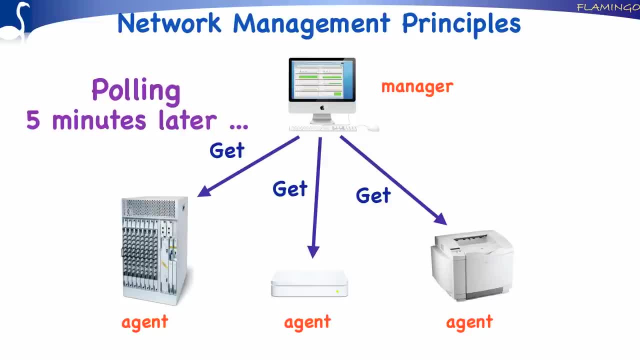 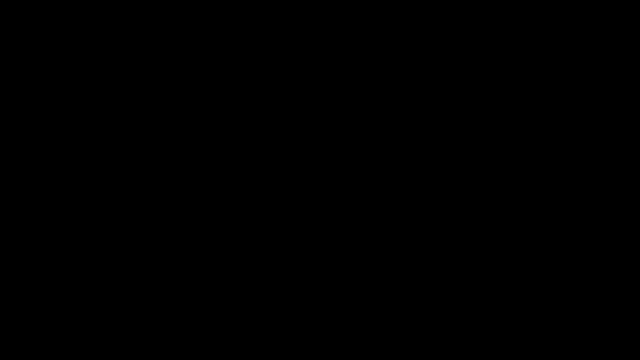 This is the cause of simplicity, as advocated by SNMP For fairness. we must say, however, that with later versions of SNMP, agents have more capabilities to report the manager of certain events, thus reducing a bit the need for polling. The last concept we'll discuss in this tutorial. 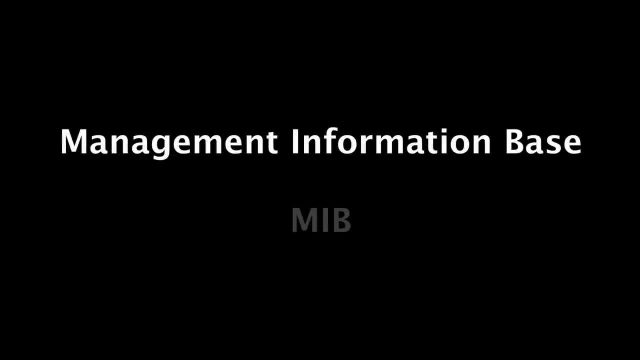 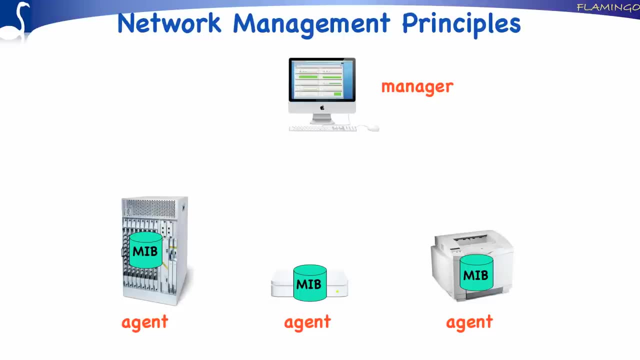 is the management information base, the MIB. MIBs are included in every agent and organized in a way that allows for a more precise and accurate analysis of the agent. The management information base is divided into so-called MIB modules. Some of these modules: 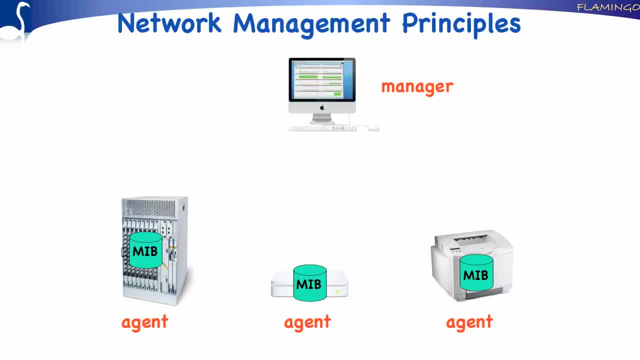 are implemented in every agent, since they hold generic information applicable to all devices, for example the IP address of the device or the time the agent is up. Other modules are only implemented in certain kinds of devices, since they hold information specific for that particular kind of device. 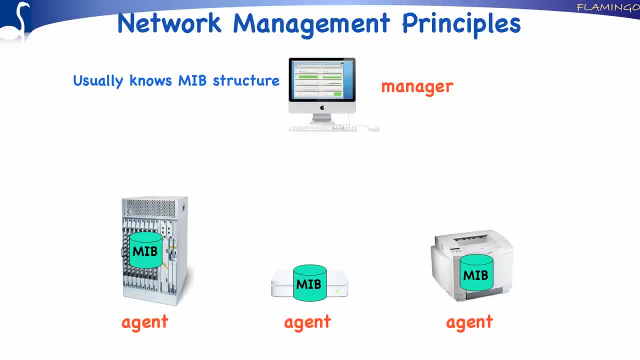 such as the IP address of the device. The manager usually knows the MIB structure of the various agents, thus which management information is maintained by each agent. In addition, managers usually store previously retrieved management information to detect, for example, anomalies or to plot a router's outgoing traffic.